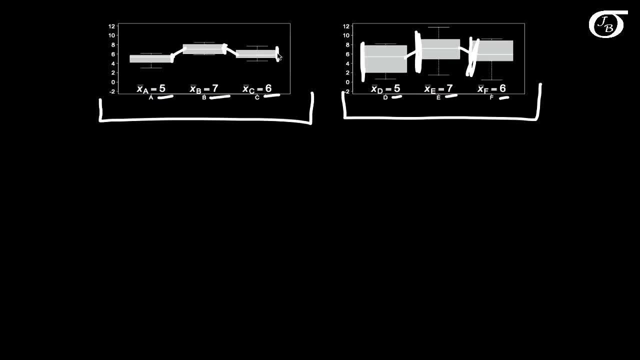 So there is greater variability within groups here than over on the left. Let's see what the end result of an analysis on the left looks like. Let's see what the end result of an analysis on the left looks like. We will learn how to carry out this test as we go along. 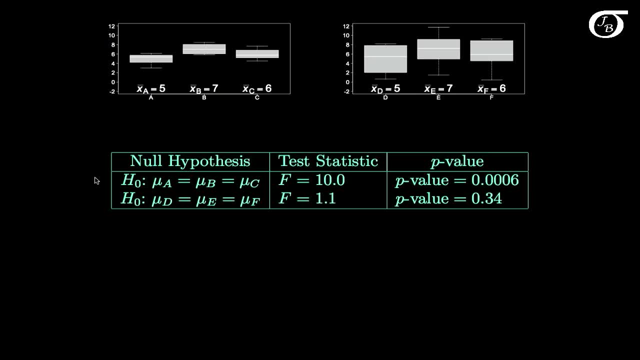 But if we know something about hypothesis testing and we know what the null hypothesis is and we can properly interpret a p-value, we should be able to see here that for this null hypothesis that muA and muB and muC are equal. 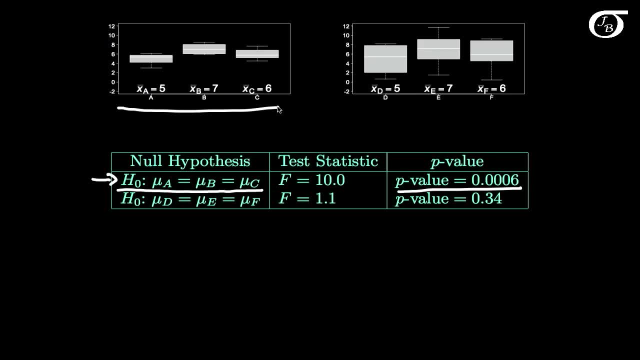 or in other words, that these three samples come from three populations that all have the same population mean the p-value is very, very small. The p-value is very, very small over here. So there is very strong evidence against this null hypothesis. We'll see. this test statistic is an F test statistic. 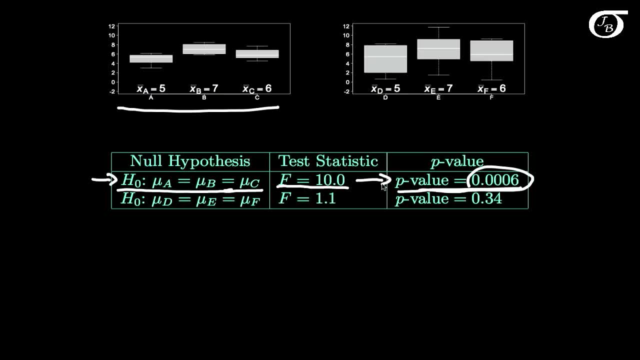 and that F test statistic is going to help us get this p-value. But for now we can look at this p-value and say there is very strong evidence against that null hypothesis. But if we look at the other side, corresponding to the plot on the right, 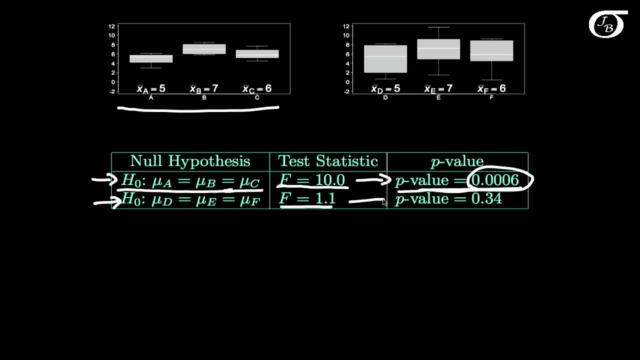 we'd see that our F statistic is rather small, yielding a large p-value. So we get a large p-value here, meaning that there is not strong evidence against this null hypothesis. Note again that the only difference between these two scenarios is that the variability within groups on this side is much greater than over here. 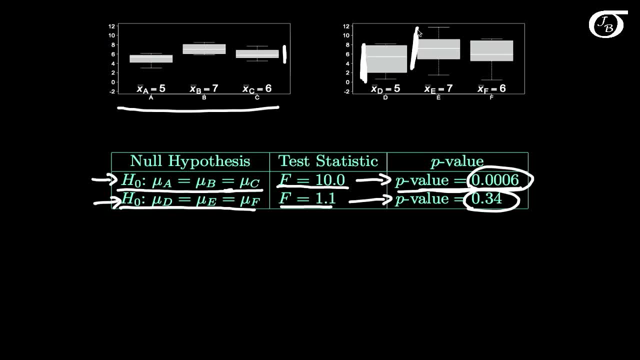 What happened then is that the variability within the groups over here swamped the variability between the groups and we didn't see a significant difference. And, to summarize, the p-values tell us that there is strong evidence against the null hypothesis that muA and muB and muC are equal. 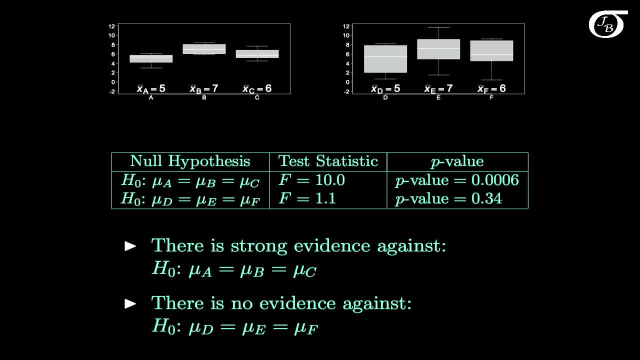 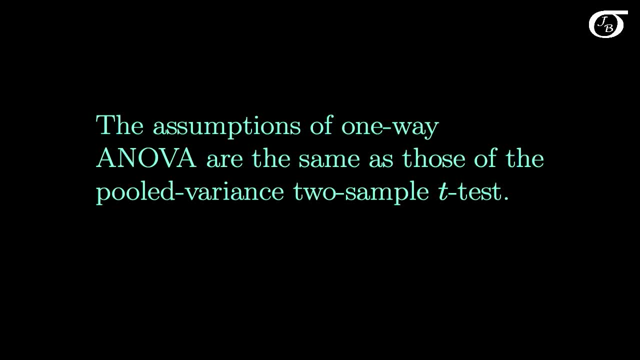 but there is no real evidence against the null hypothesis that muD E and F are equal. One-way analysis of variance can be viewed as a generalization of the pooled variance two-sample t-test to more than two groups And, as such, the assumptions of one-way analysis of variance. 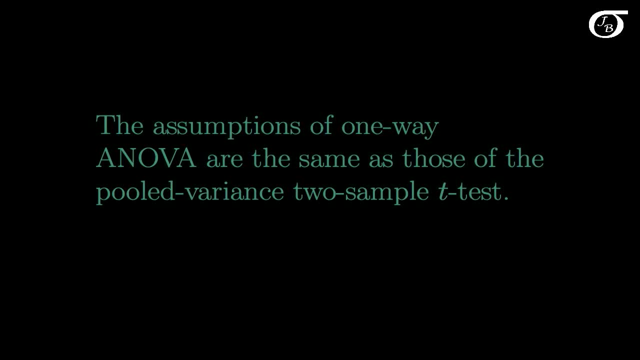 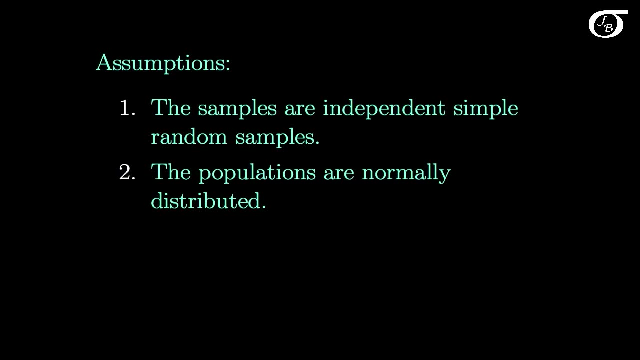 are the same as those of the pooled variance two-sample t-test. Specifically, we are assuming that we have independent, simple, random samples, that the populations are normally distributed and that the population variances are equal. Or, in other words, sigma1 squared through sigma k squared are all equal.